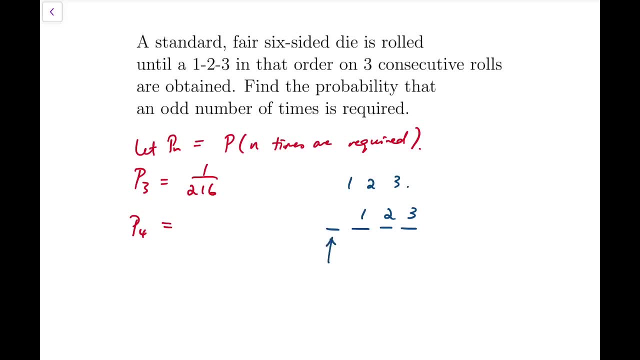 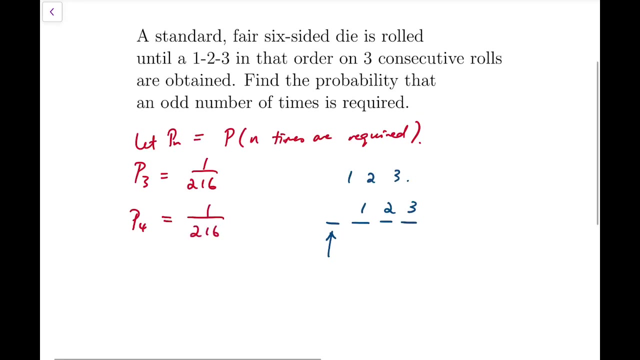 over 233.. Now the result of the first roll. it can be anything, because no matter if it's 123456, it will not affect the outcome. You still need 4 rolls anyway. So the probability is still 1 over 216.. 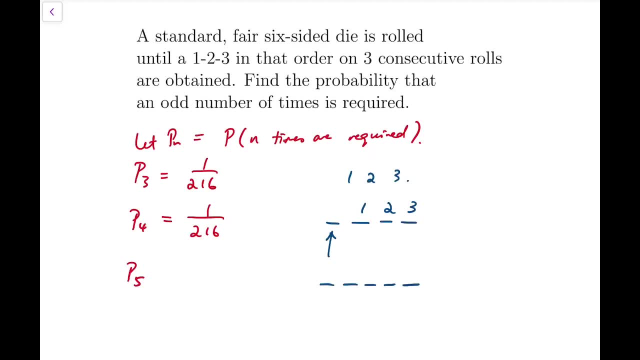 And that's similar for the case that we need 5 times, because once we have fixed the last 3 rolls, the result of the last 3 rolls 123.. And these 2 could be anything, No matter. regardless of the combination, we will not. 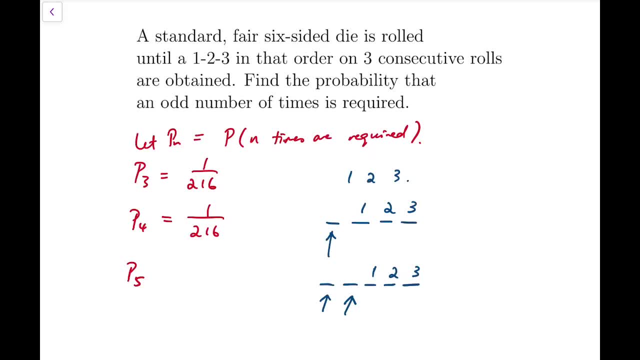 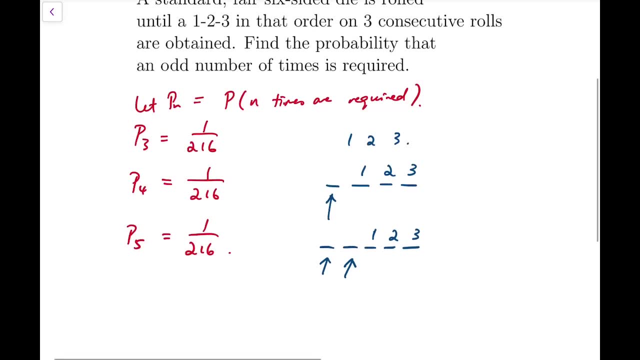 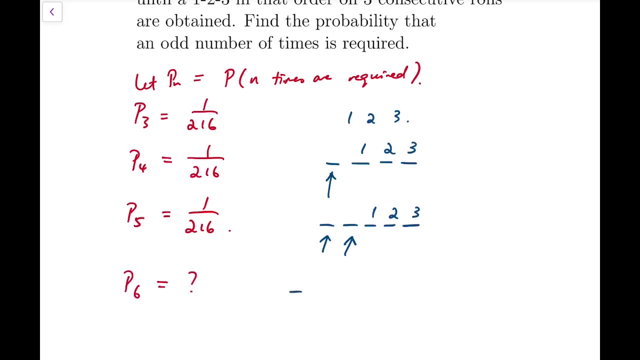 get 123 earlier than the 5th roll, So it's still 1 over 216.. However, when it comes to 6 rolls, things go a bit different, Even with a fixed roll, In other words- so we fixed the last 3 rolls- there's still a possibility. 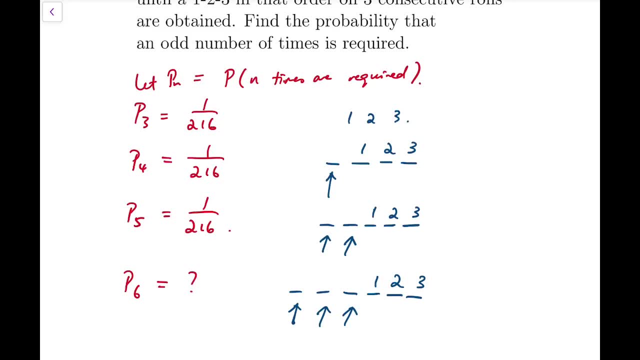 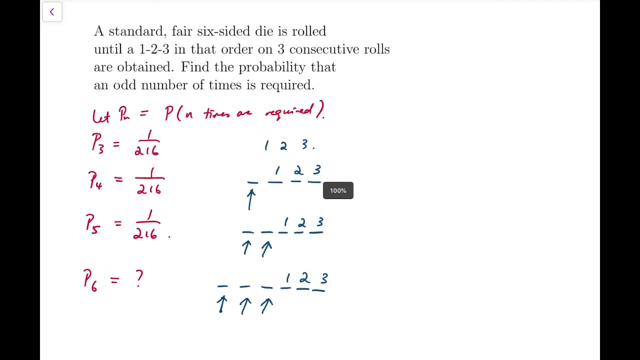 for us to achieve this earlier than the 6th roll, which is that we have exactly 123 at the first 3 rolls. So things just start to get a bit out of control, but it's still manageable. Another point that I would like to make is that whenever those kinds of problems turn up within a rotation, 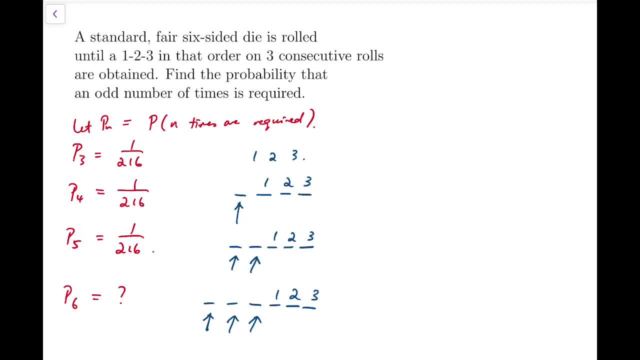 the concept of recursion would definitely come into play. The reason is that this kind of a situation applies to infinitely many number of rows, Say, we still have to take into account on, say, a thousand and one rows, or even a million and one rows. 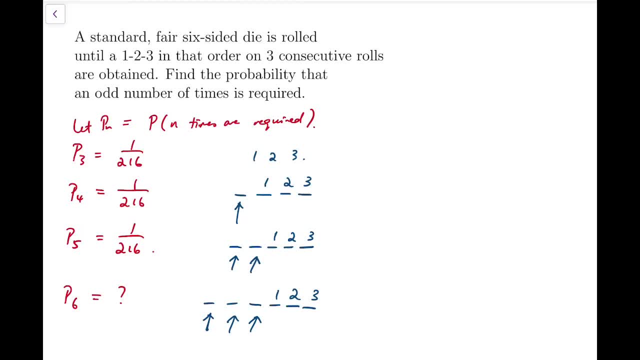 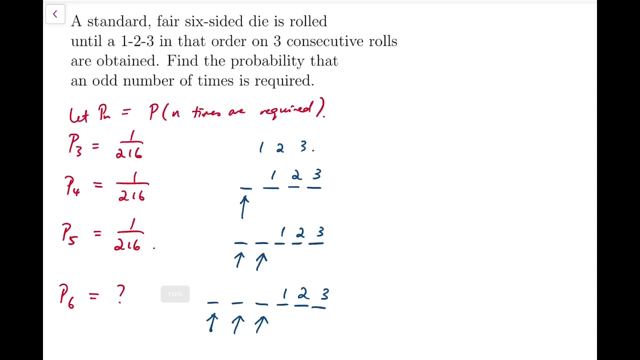 But it's impossible for us to calculate all of them, So we have to look for some pattern that helps us to investigate what would happen when the number of rows gets larger and larger, And so here's an observation: It's that when the number of rows turns to six from five, 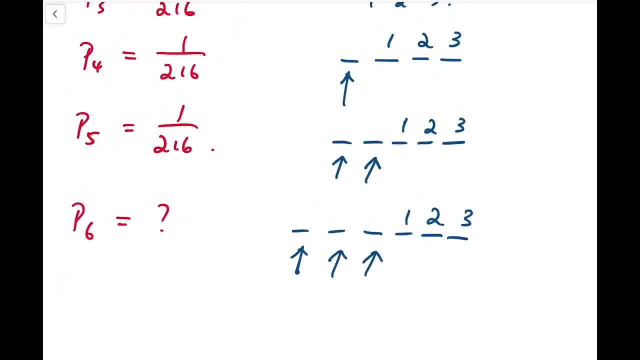 from five to six. you can see that, apart from adding an extra row, there's actually a kind of bijection between each of the possibilities under five rows and some of the possibilities under six rows. It's that it's just a direct copy of the cases in P5,. 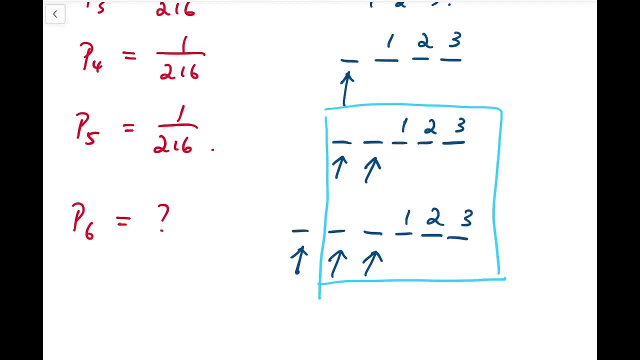 and then we add an extra number at the very left of that string. However, there is one special case that we have to take it out is that if the first two rows under the cases in P5 are two and three, so write two and three here. 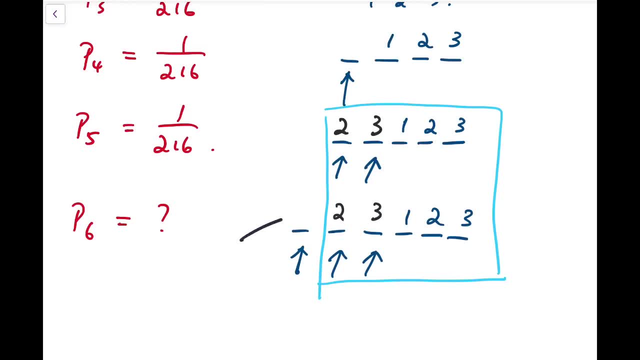 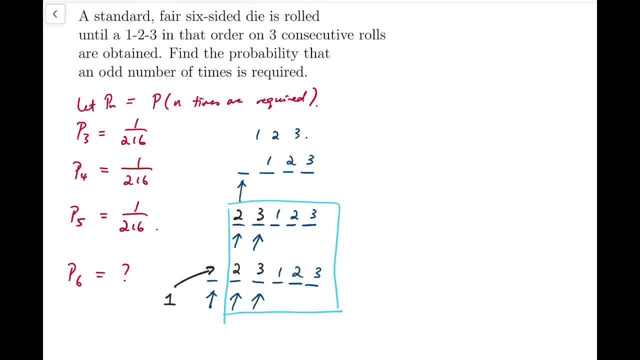 and we directly copy and if the first row we get one in the first row under the cases in P6, then that will not work. So in fact I can claim that P5 is actually just. there's only a slight difference between P5 and P6,. 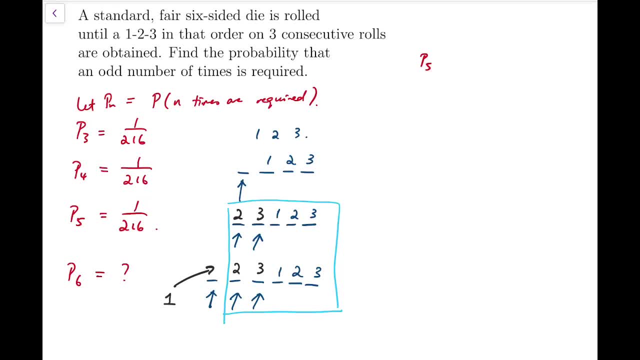 which is that we can directly copy all cases in P5 to P6, but we have to take out this one, two, three case, one of the cases in P6, and that's in a kind of, in a kind of a. 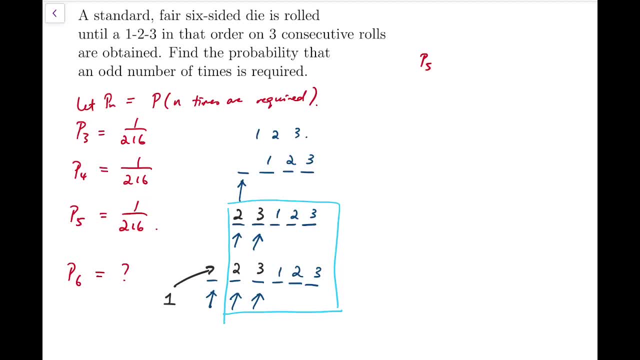 a ratio of 1 over 216. and so from that argument we know that p5 should be slightly larger than p6. so we can subtract that and we know that we have to take out 1 over 216 of the cases in p6. so that's 1 over 216 times p, we're. 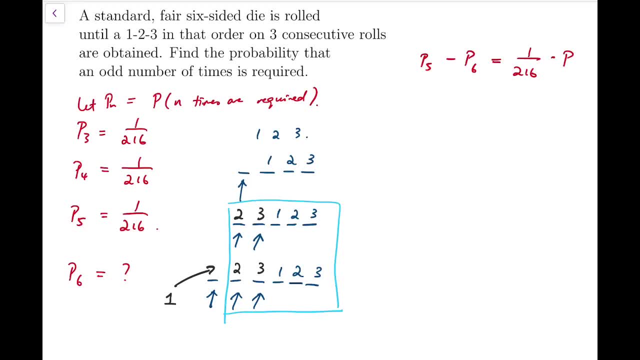 not exactly p6, but p3 instead, because we are multiplying these cases- okay, the cases under p3- by an extra 1 over 216, which is what happens, what exactly happens in the previous three rows of those within a red circle. so it becomes 1 over 216 times p3 and in fact we can actually do something. 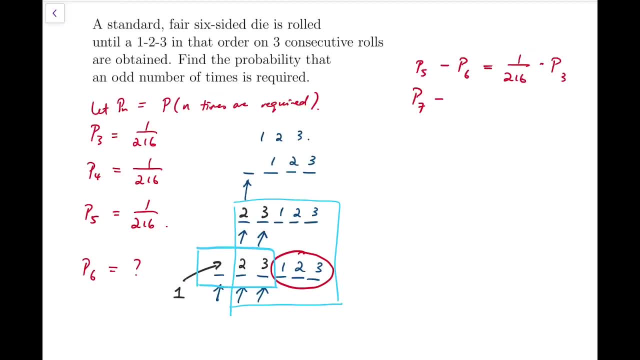 similar for, say, p7 minus p8, and that's again 216 times. and looking at the pattern, that should be p5, because what happens in the red circle could be arbitrarily lost and the number of rows inside the red circle could be arbitrarily large. so we 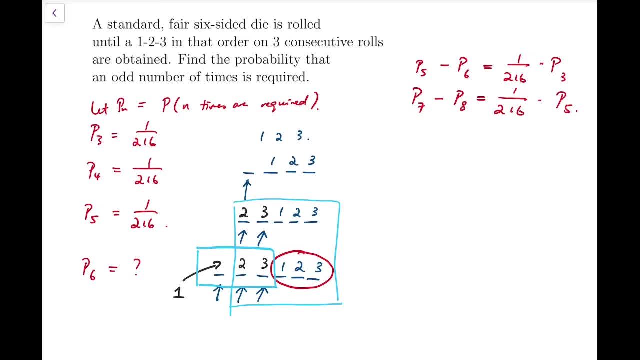 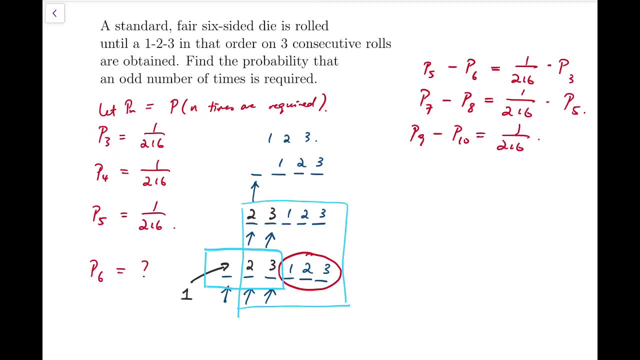 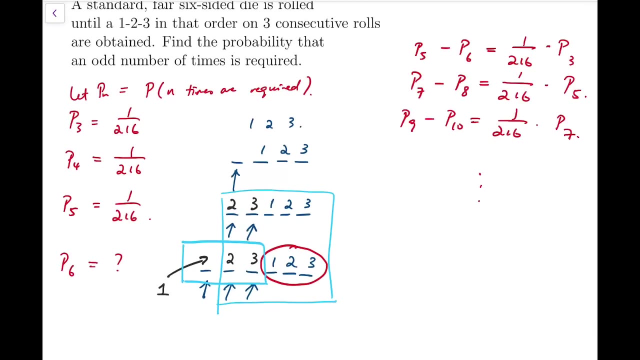 can keep looping this, iterating this with bigger cases. say, p9 minus p10 equals 1 over 216 times p7, and so on. now notice that all of these terms- okay, the first terms under these recurrence relations are other cases that odd number of times are required and the green cases. 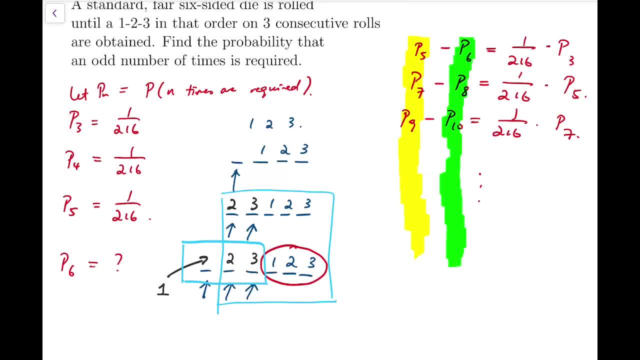 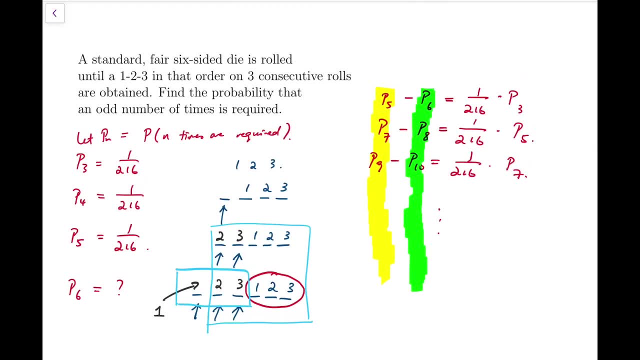 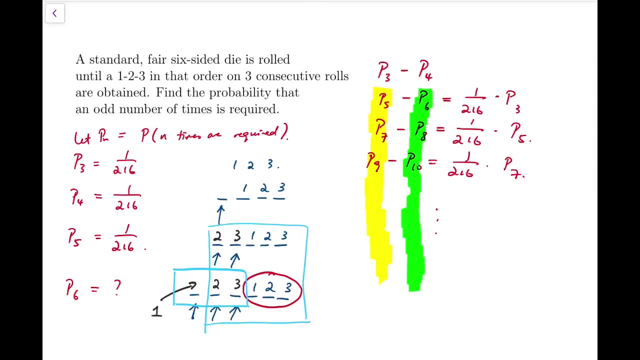 okay, the second terms okay in each in each recurrence relation are the even cases, so we can actually add them up and together with another similar equation, which is that p3 minus p4. so to make the whole thing more complete, however, p3 minus p4 is actually zero from our 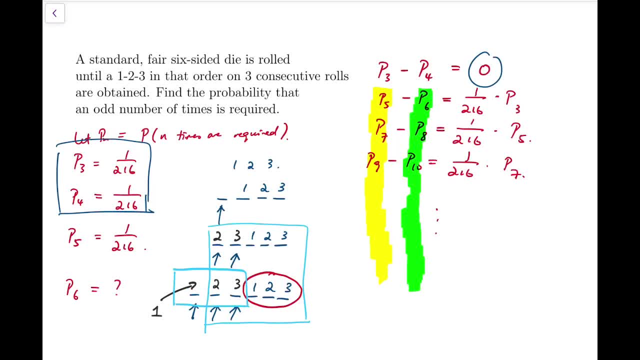 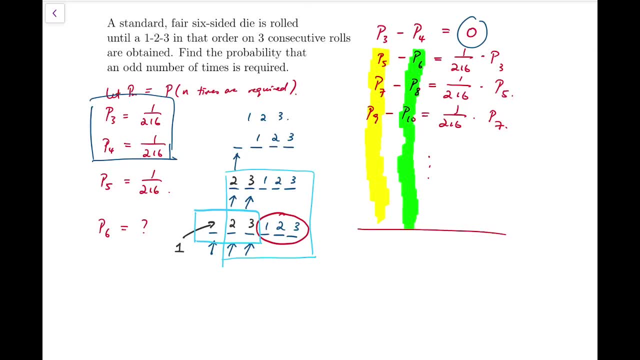 previous calculations we have actually got that, so that's zero. now we add them all up. so after adding we will get p, say p odd, and then minus p even equals to 1 over 216 times p odd. now we can further simplify by rewriting P even actually into P odd, because the